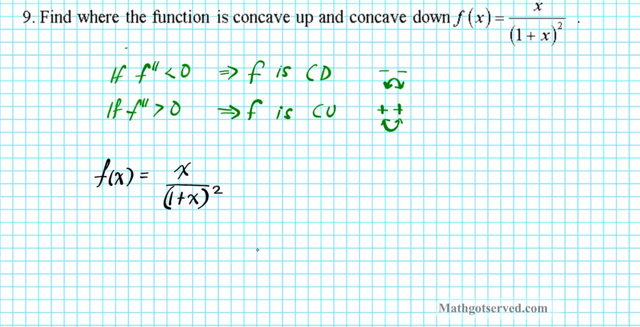 All right now, if we try to solve the problem, all of these problems will come down as plus ah and the result of all our other rules. here. This is Y, essentially times, and the exact valuelection to our usual wasn't the solution, but we try to find the first derivative. where the other three can only beestic. This equation can be used with a number. All right, this is the first derivative we already have here. If the foreign derivative is posit, then substituting the positive elimination, it's posit. Thevl bin is: look, it's not the non engagement- 15 singver. 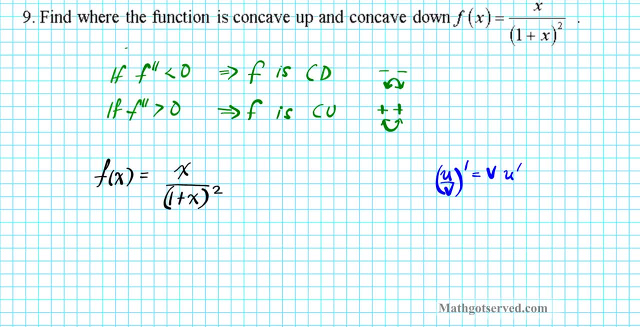 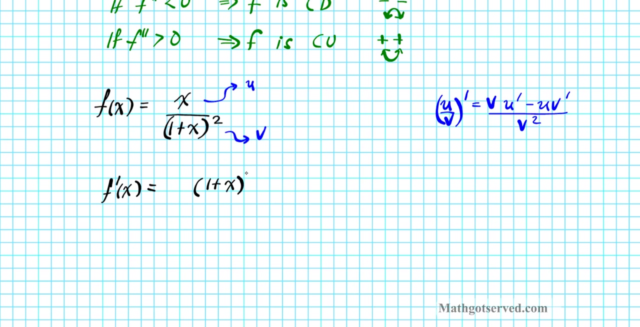 is equal to v: u prime minus u, v prime, okay, divided by v square. so in this problem um x is u and the denominator one, the quantity one plus x square is v. all right, so f prime. the first derivative is going to be v, which is one plus x quantity square times the derivative of x. 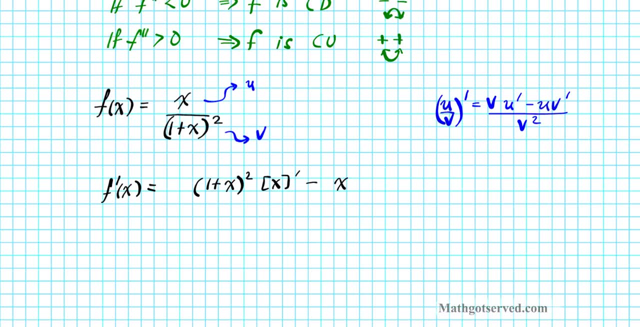 minus u, which is x times uh, the quantity. one plus x square prime. all right, and then that's uh u v prime, and then we divide that by v square, so we'll have um one plus x quantity square square. all right, let's go ahead and differentiate. 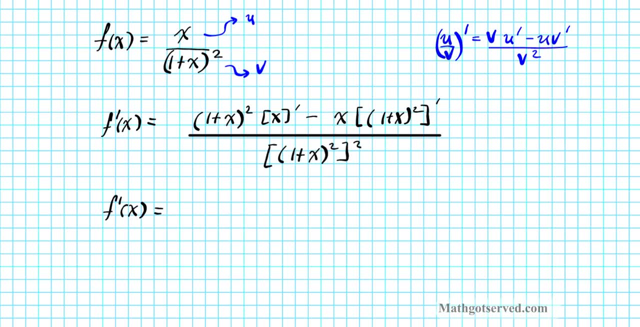 uh, we have f. prime of x equals one plus x quantity square. now, um x prime is just one, and then times one minus x. now, when we are differentiating one plus x quantity square, we're going to be using the chain rule. so we're going to be using the chain rule. the outer function here is x square, its derivative is 2x, and the inner function is one plus x and its derivative is just one. so we're going to evaluate the derivative of the outer function at the inner function. so we're going to take this and plug it in there and then multiply it by the derivative of the inner function. okay, so, applying the chain rule here, we're going to have times two times one plus x to the first power and then we're going to multiply it by the derivative of the inner function. okay, so, applying the chain rule, here, we're going to have times two times one plus x to the first power and then we're going to multiply it by the derivative of the inner function. okay, so, applying the chain rule here, we're going to have times two times one plus x to the first power and then we're going to multiply it by the derivative of the inner function. okay, so, applying the chain rule here we're going to have times, two times one plus x to the first power, and then we're going to multiply it by the derivative of the inner function. 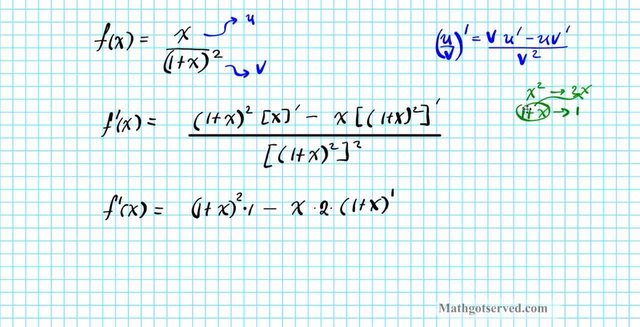 that is the derivative of the outer function, x square evaluated at the inner function, one plus x times the derivative of the inner function, which is just one. okay, all right. and then we're going to divide this by the square of the denominator, using the power of a power property. we're going 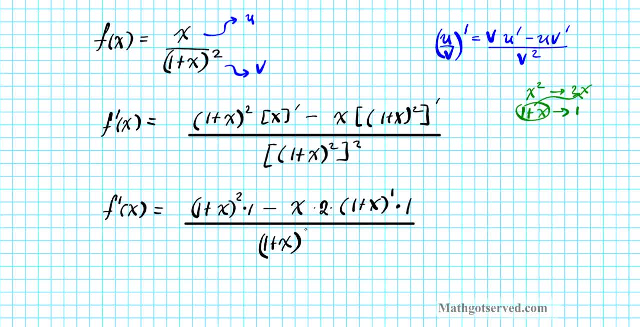 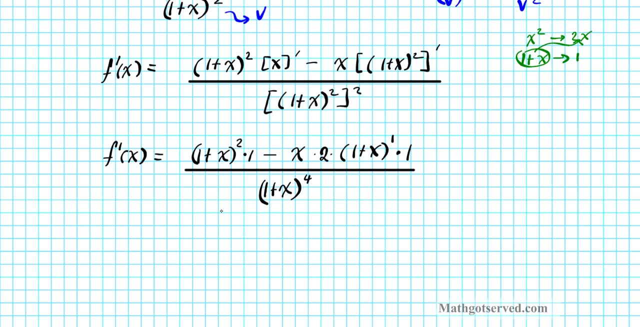 to have one plus x quantity raised to the fourth power. okay, you just multiply the exponents whenever you raise the power to a power. all right, let's simplify it a little bit more. so we're going to have a one plus x square. so simply one plus two x plus one minus. we'll distribute two x to this. 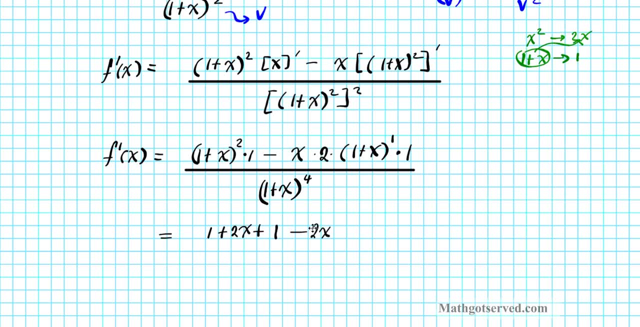 quantity here and we'll have negative two x minus two x square. okay, let's see, make a real quick correction here. this is plus x square. all right, so we have the numerator expanded out completely. let's see if we can combine uh like terms. so in the numerator um the two x's, two x and negative two x add up to zero. 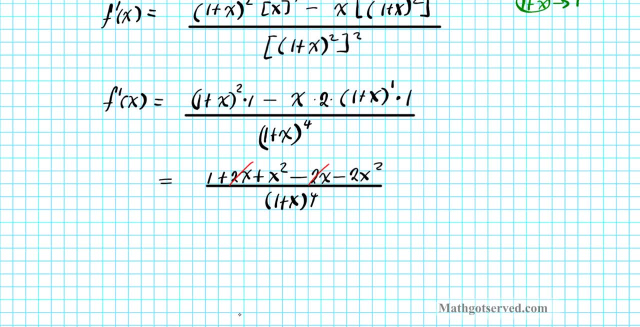 so now we are going to have: uh, let's see f prime of x. f prime of x is equal to one um x square minus two x square is negative x, negative um x square and we have that divided by one plus x to the fourth, one plus x to the fourth. 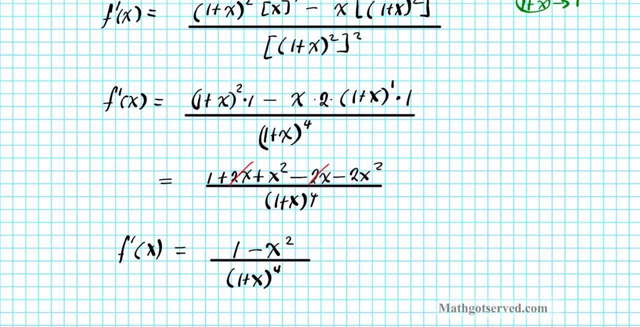 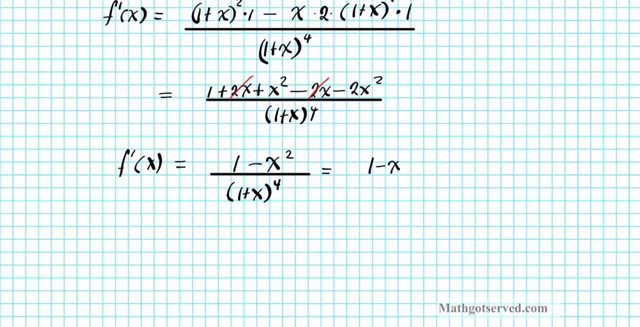 here we can. here we can factor it right. we can factor it into one minus x factor it right. we can factor it into one minus x factor it right. we can factor it into one minus x times one plus x times one plus x times one plus x, and we'll divide that by um. 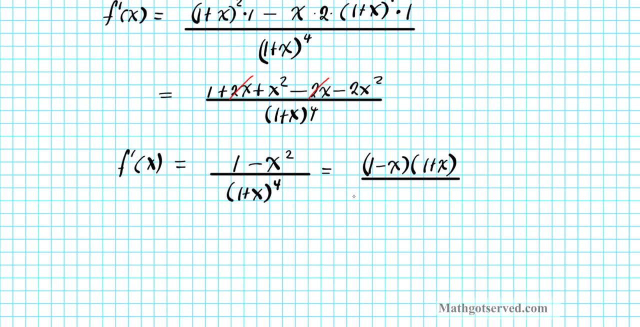 and we'll divide that by um, and we'll divide that by um: one plus x to the fourth, one plus x to the fourth, one plus x to the fourth. so you can see that, uh, we can make a. so you can see that, uh, we can make a. 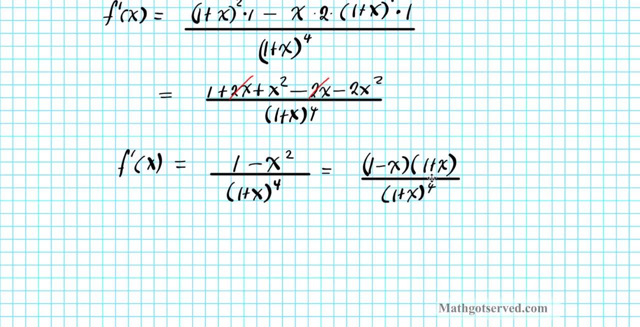 so you can see that, uh, we can make a reduction here, reduction here, reduction here, we can reduce this, we can cancel out on, we can reduce this, we can cancel out on, we can reduce this, we can cancel out on this in this one plus x to the fourth. 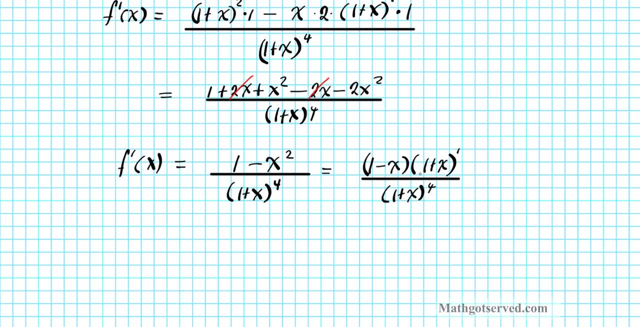 this in this one plus x to the fourth, this in this one plus x to the fourth, with a one plus x to the first power in with a one plus x to the first power in, with a one plus x to the first power in the numerator, the numerator. 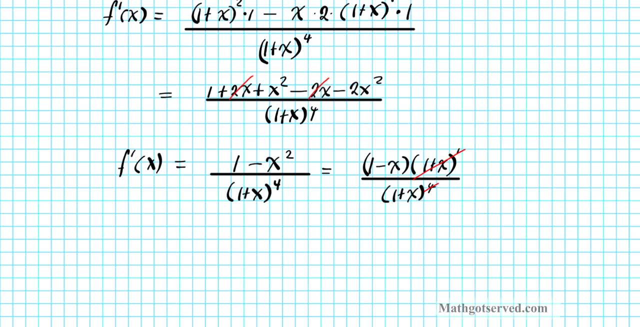 the numerator. okay, so this. you just subtract the. okay, so this. you just subtract the. okay, so this: you just subtract the exponents. this gets reduced by one exponents. this gets reduced by one exponents. this gets reduced by one to three. okay, so we have to three. okay, so we have. 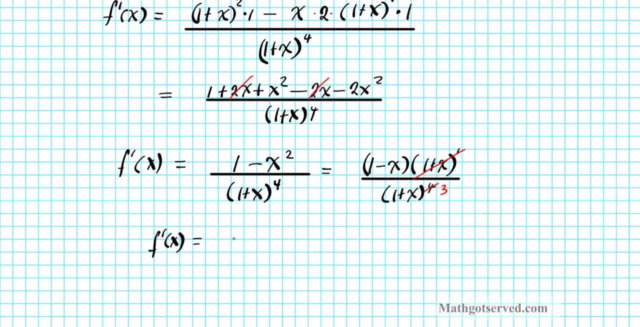 to three. okay, so we have f prime of x equals f. prime of x equals f prime of x equals uh. one minus x. uh, one minus x. uh, one minus x over over over. one plus x to the third, one plus x to the third, one plus x to the third. okay, now, what are we going to do? 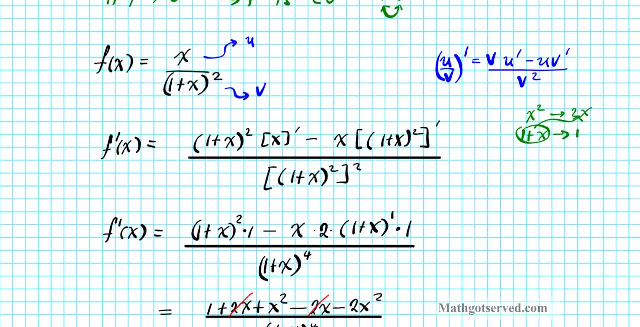 okay now, what are we going to do? okay now, what are we going to do next? well, let's go back to the beginning next. well, let's go back to the beginning next. well, let's go back to the beginning. remember, we said remember. we said remember. we said: to find the concavity we need to look at. 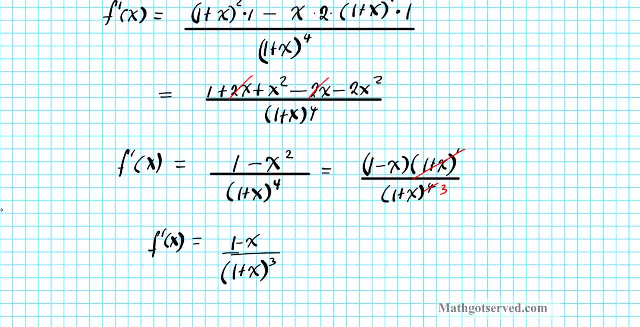 to find the concavity we need to look at. to find the concavity, we need to look at the sign of the second derivative. the sign of the second derivative, the sign of the second derivative. okay, what do we have? we have the first. okay, what do we have? we have the first. 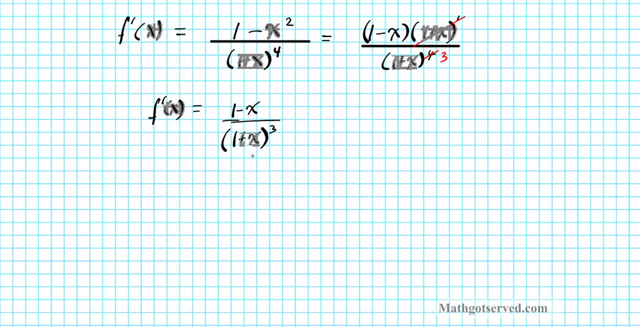 okay, what do we have? we have the first derivative, derivative, derivative. so we're going to do what we're going to. so we're going to do what we're going to, so we're going to do what we're going to: differentiate again, differentiate again, differentiate again. all right now, um, we're going to use the. 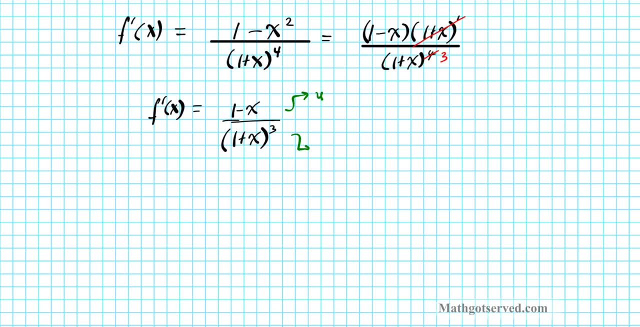 all right now. um, we're going to use the all right now. um, we're going to use the quotient rule again. this is u quotient rule again. this is u quotient rule again. this is u. the numerator and the denominator is v. the numerator and the denominator is v. 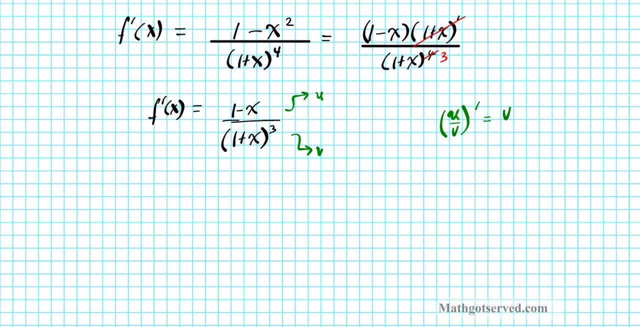 the numerator and the denominator is v. remember what the quotient rule is. u remember what the quotient rule is? u remember what the quotient rule is? u over v prime is equal to v. u prime over v prime is equal to v. u prime over v prime is equal to v. u prime minus. 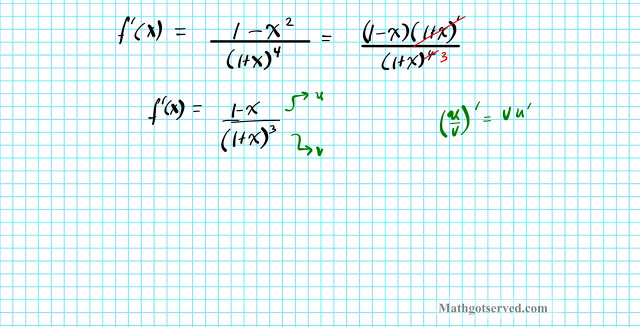 minus minus, so v? u prime minus u v prime divided by v square, divided by v square, divided by v square. all right, so let's go ahead and apply. all right, so let's go ahead and apply. all right, so let's go ahead and apply that here. 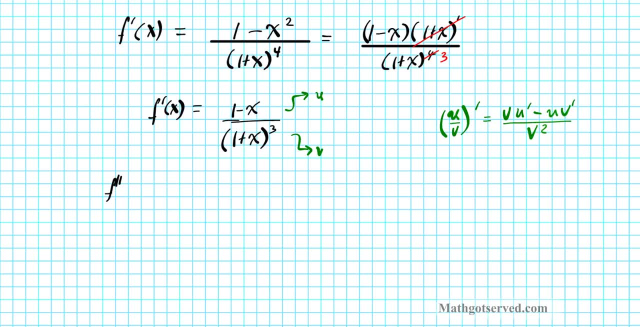 that here. that here. so the second derivative f double prime, so the second derivative f double prime. so the second derivative f double prime of x is equal to v, of x is equal to v, of x is equal to v, which is 1 plus x to the third. 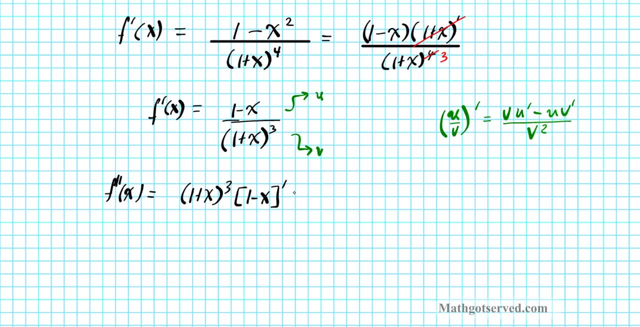 which is 1 plus x to the third, which is 1 plus x to the third. times u prime 1 minus x. times u prime 1. minus x. times u prime 1 minus x. prime minus u, which is quantity 1 minus x. prime minus u, which is quantity 1 minus x. 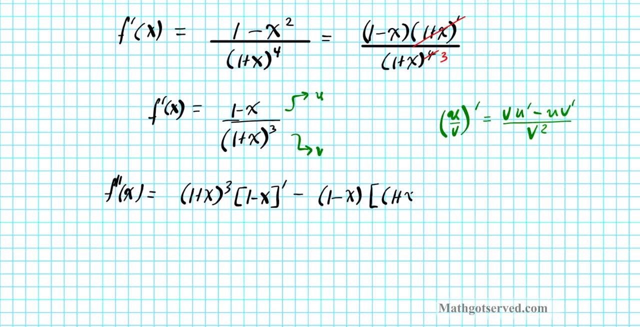 prime minus u, which is quantity 1 minus x times times times v. prime, which is 1 plus x. quantity v prime which is 1 plus x. quantity v prime, which is 1 plus x. quantity raised to the third. raised to the third. raised to the third prime divided by: 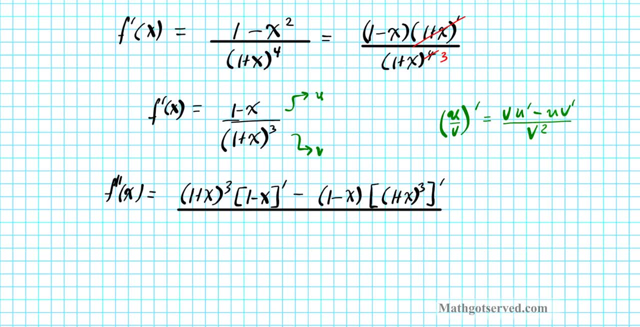 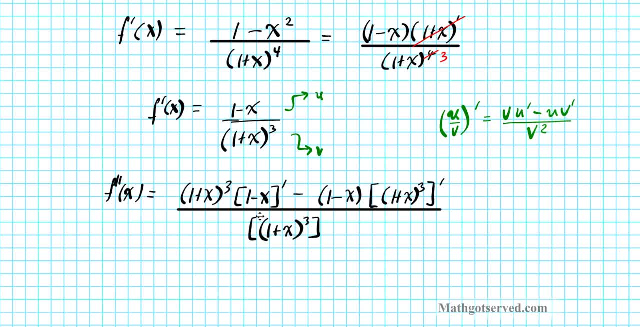 be 1 plus x. raised to the third. raised to the third. raised to the third. square the entire quantity. okay, square the entire quantity. okay, square the entire quantity. okay, all right. so that's how we'll find the all right. so that's how we'll find the. 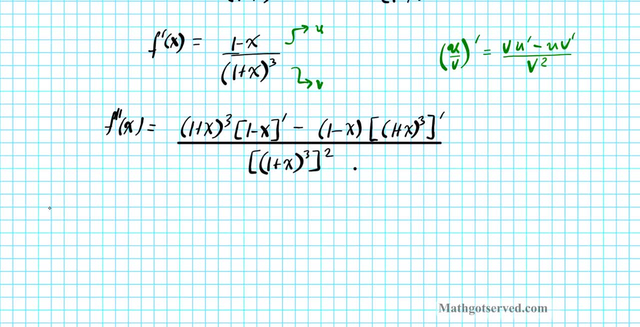 all right, so that's how we'll find the second derivative, second derivative, second derivative. so let's go ahead and differentiate, and so let's go ahead and differentiate, and so let's go ahead and differentiate, and then simplify, then simplify, then simplify. f double prime of x is equal to. 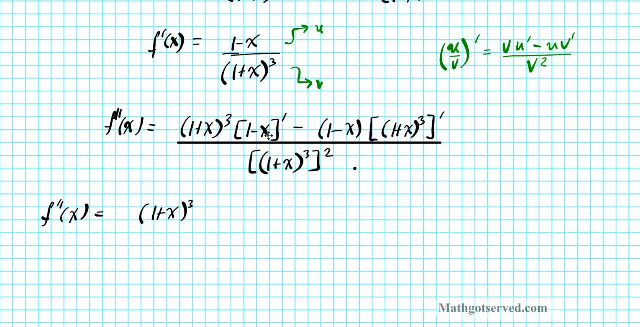 f. double prime of x is equal to f. double prime of x is equal to 1 plus x to the third. now the derivative 1 plus x to the third, now the derivative 1 plus x to the third, now the derivative of this is just, uh, negative 1. 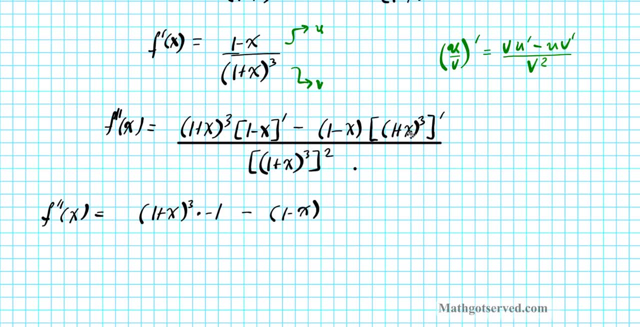 of this is just uh negative. 1 of this is just uh negative: 1 minus minus minus 1 minus x. we're going to apply the chain 1 minus x. we're going to apply the chain 1 minus x. we're going to apply the chain rule here again. 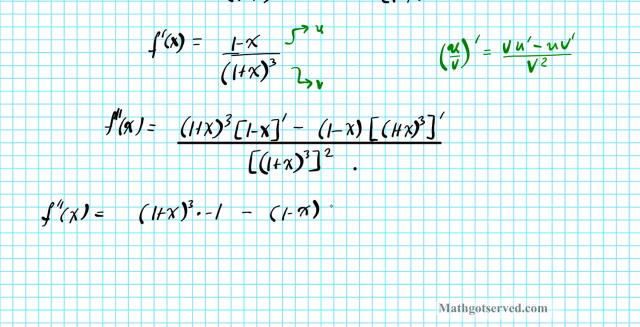 rule here again, rule here again: differentiate the outer function which differentiate the outer function, which differentiate the outer function which is x to the third, is x to the third, is x to the third. it's going to be 3x squared, so we have. it's going to be 3x squared, so we have. 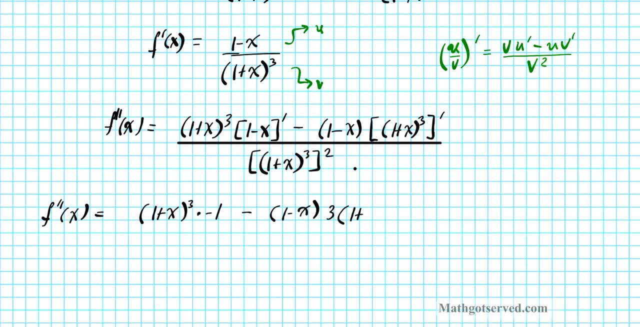 it's going to be 3x squared. so we have three times instead of x, three times instead of x, three times instead of x. we plug in the inner function, which is: we plug in the inner function, which is: we plug in the inner function, which is 1 plus x. so this is 3x squared evaluated. 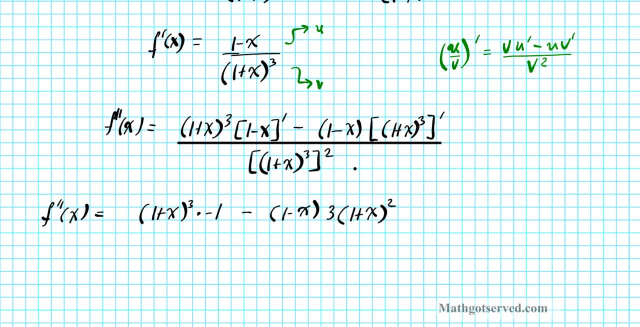 1 plus x- squared 1 plus x. 1 plus x- squared 1 plus x. 1 plus x squared 1 plus x. all right, so, all right, so all right. so we have that and then we multiply it of. we have that and then we multiply it of. 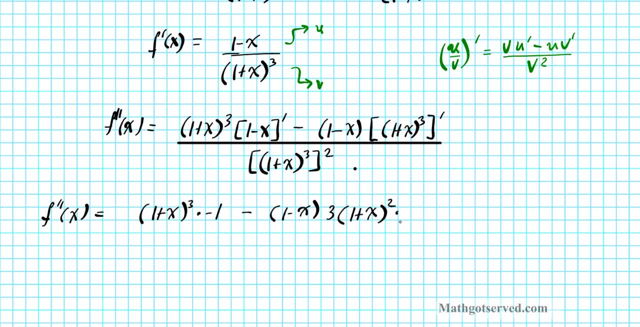 we have that, and then we multiply it, of course, by the derivative course, by the derivative course, by the derivative of the inner function um, which is just of the inner function um, which is just of the inner function um, which is just. derivative of 1 plus x is 1. 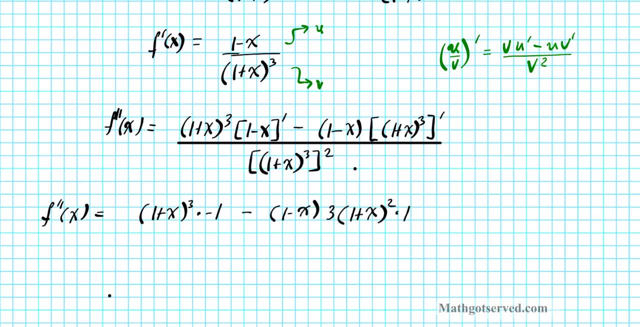 derivative of 1 plus x is 1. derivative of 1 plus x is 1. all right, so we have that divided by all right. so we have that divided by all right. so we have that divided by the denominator square, the denominator square, the denominator square. so. 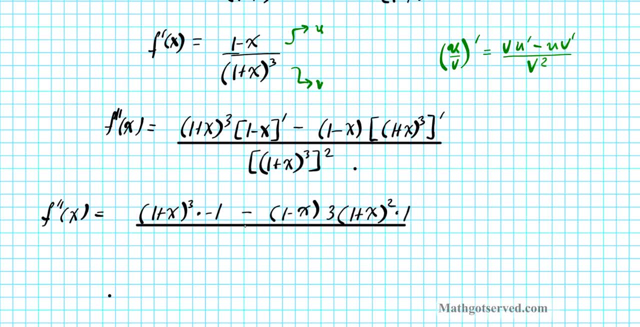 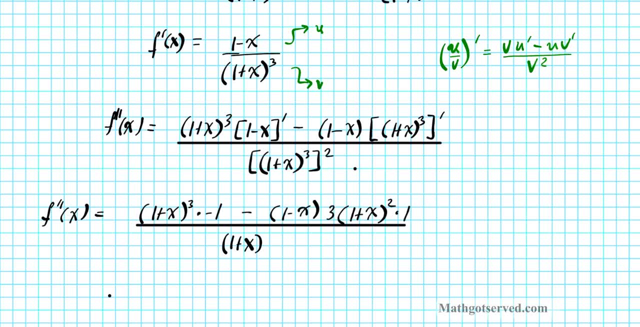 actually, let's just simplify that we actually let's just simplify that we just multiply the powers, so 3 times 2, just multiply the powers, so 3 times 2. just multiply the powers, so 3 times 2 is 6. is 6.. 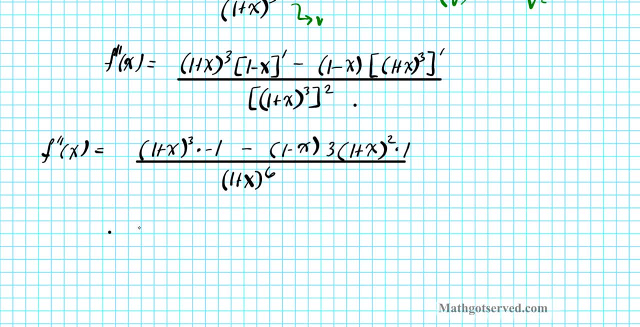 is 6.. okay, now we're done differentiating. okay, now we're done differentiating. okay, now we're done differentiating. let's go ahead and simplify. let's go ahead and simplify. let's go ahead and simplify. now, if you notice, i have a 1 plus x to. 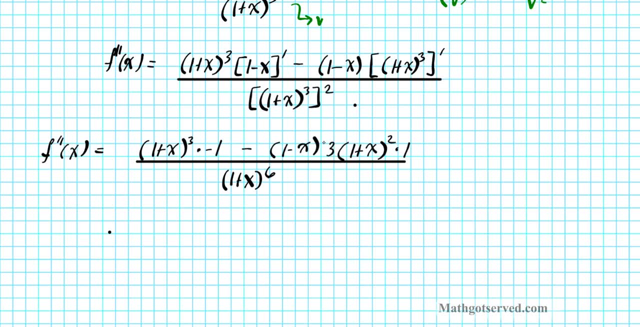 now, if you notice, i have a 1 plus x to now. if you notice, i have a 1 plus x to the third here and a 1 plus x squared the third here and a 1 plus x squared the third here and a 1 plus x squared, so i can factor out the gcf. 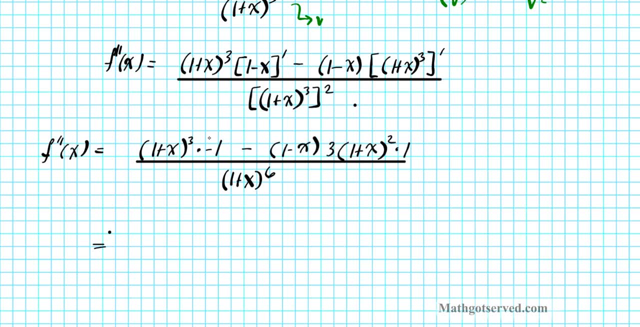 so i can factor out the gcf. so i can factor out the gcf which is 1 plus x to the second power, which is 1 plus x to the second power, which is 1 plus x to the second power, the smaller of the two factors, with: 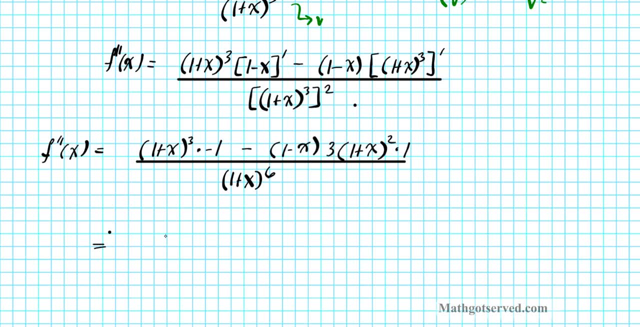 the smaller of the two factors, with the smaller of the two factors with identical, identical, identical bases. okay, so we have bases. okay, so we have bases. okay, so we have 1 plus x to the second power, 1 plus x to the second power, 1 plus x to the second power, and then we're left with- let's not. 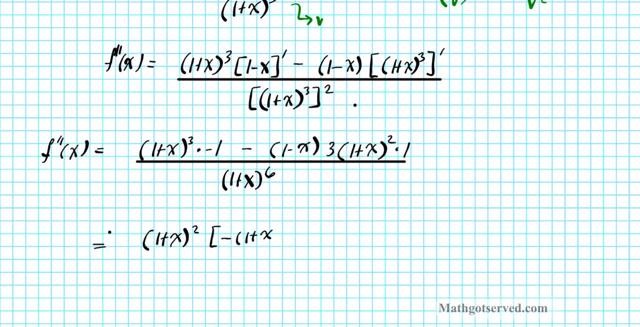 and then we're left with let's not. and then we're left with: let's not. forget this minus, forget this minus, forget this: minus negative: 1 plus x, and then minus negative: 1 plus x, and then minus negative: 1 plus x, and then minus 3 times 1 minus x. 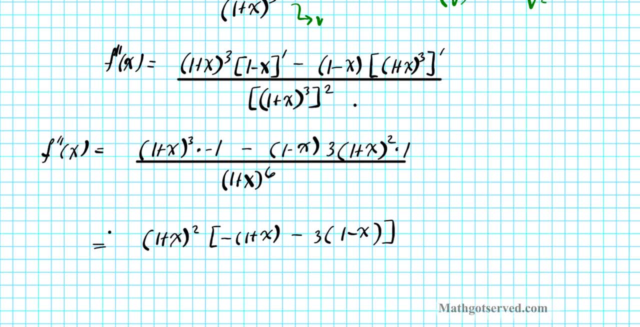 3 times 1 minus x, 3 times 1 minus x. okay, okay, okay. and then we'll divide by, and then we'll divide by, and then we'll divide by 1 plus x to the sixth. all right now, you notice that these can. all right now, you notice that these can. 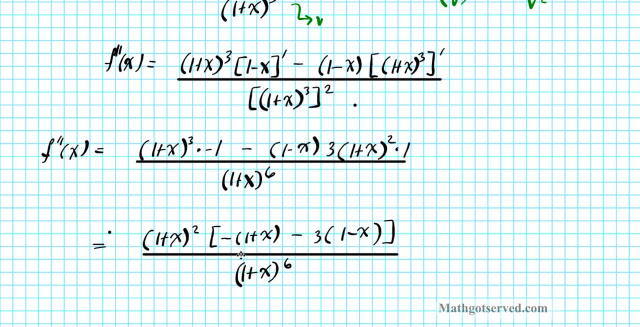 all, right. now you notice that these can be reduced, right? you just simply be reduced, right? you just simply be reduced, right. you just simply subtract the exponents using the quotient. subtract. the exponents using the quotient. subtract the exponents using the quotient property of exponents. um. 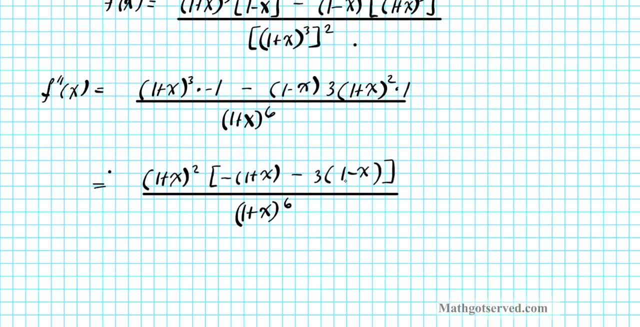 property of exponents um. property of exponents: um. and then over here we can just distribute, and then over here we can just distribute, and then over here we can just distribute, and then simplify okay, and then simplify okay, and then simplify okay. so let's go ahead and reduce this. 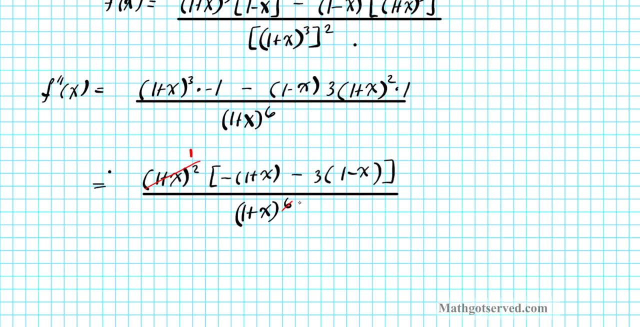 so let's go ahead and reduce this. so let's go ahead and reduce this: 1 plus x squared goes here once, and 1 plus x squared goes here once, and 1 plus x squared goes here once. and this one just reduces by. this one just reduces by. 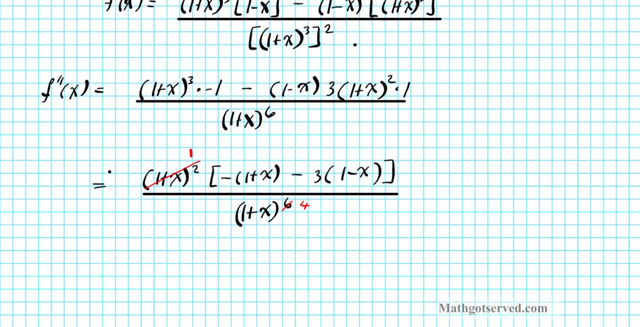 this one just reduces by 2. you subtract 2 from the power here, 2. you subtract 2 from the power here, 2. you subtract 2 from the power here, which is 4, and then we can distribute, which is 4, and then we can distribute. 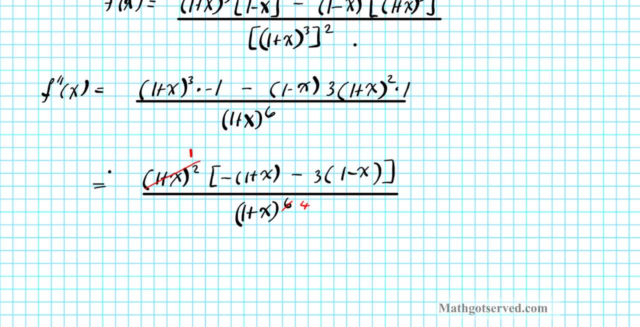 which is 4, and then we can distribute this negative 1, this negative 1, this negative 1, and then the negative 3 also. so we're, and then the negative 3 also, so we're, and then the negative 3 also. so we're going to have. 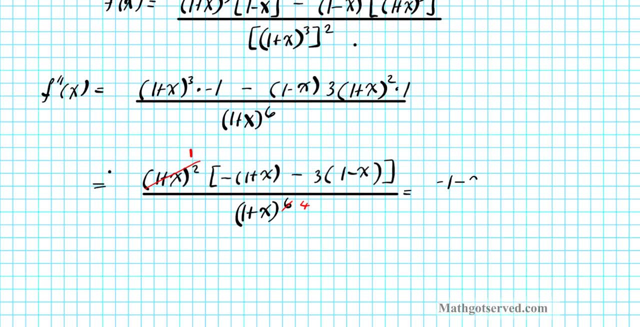 going to have. going to have um negative 1 minus x, um negative 1 minus x, um negative 1 minus x minus 3 minus 3x minus 3 minus 3x minus 3 minus 3x. okay, this becomes plus 3x. 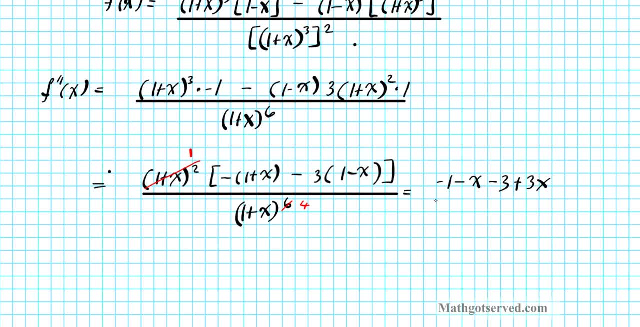 okay, this becomes plus 3x. okay, this becomes plus 3x, all right. and then that divided by all right. and then that divided by all right, and then that divided by 1 plus x to the fourth. 1 plus x to the fourth. 1 plus x to the fourth. all right, almost there, we just combine. 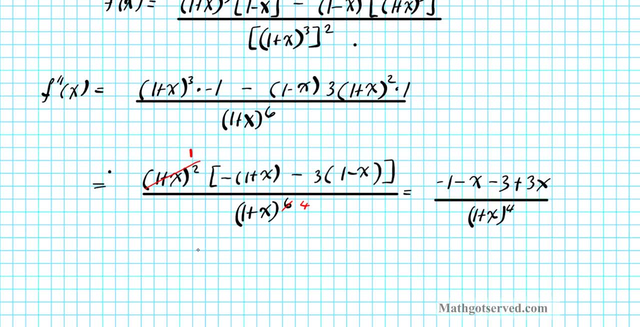 all right, almost there, we just combine. all right, almost there. we just combine like terms, like terms, like terms on the top, and that will give us the on the top, and that will give us the on the top and that will give us the second derivative. all right, so, second, 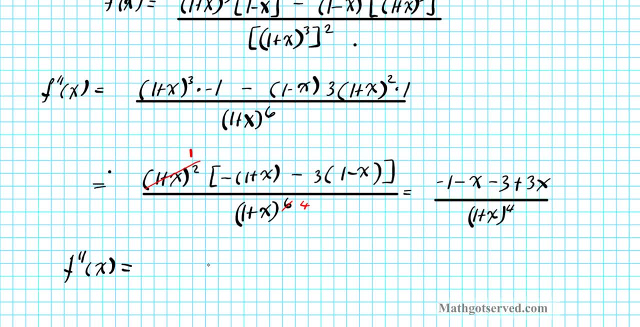 second derivative. all right, so second second derivative, all right, so second derivative of x. derivative of x. derivative of x is given by um, is given by um, is given by um. let's see what we have here. let's see what we have here. let's see what we have here: 2x minus x plus 3x is 2x. 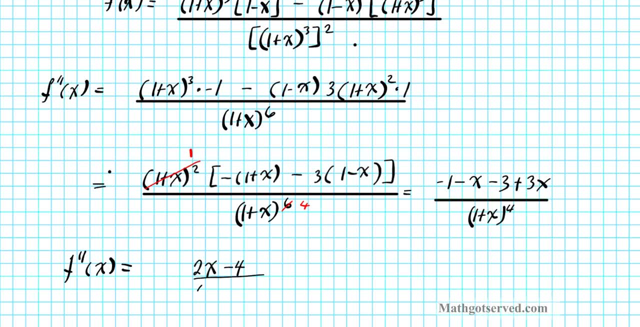 2x minus x plus 3x is 2x. 2x minus x plus 3x is 2x minus 4 divided by minus 4. divided by minus 4. divided by 1 plus x to the fourth: 1 plus x to the fourth. 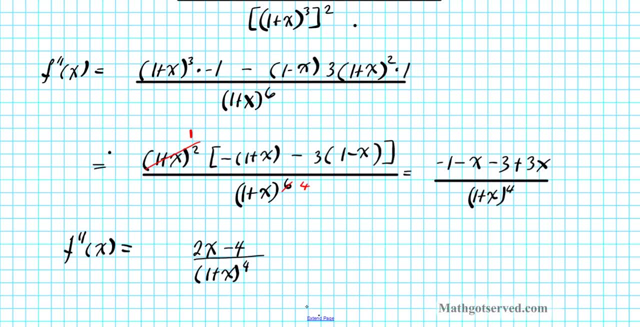 1 plus x to the fourth. all right, so now what we're going to do. all right, so now what we're going to do. all right, so now what we're going to do. we're going to look for where the second. we're going to look for where the second. 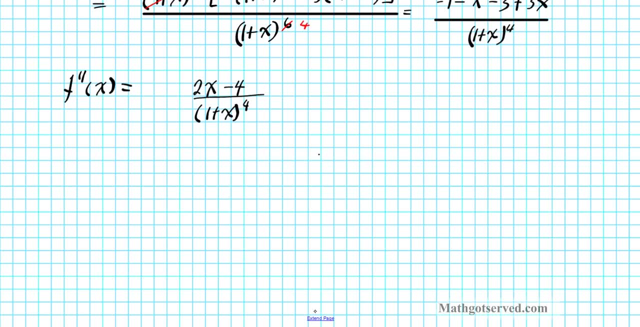 we're going to look for where the second derivative is zero derivative is zero. derivative is zero or does not exist, and then we're going or does not exist, and then we're going or does not exist, and then we're going to use that to set up. 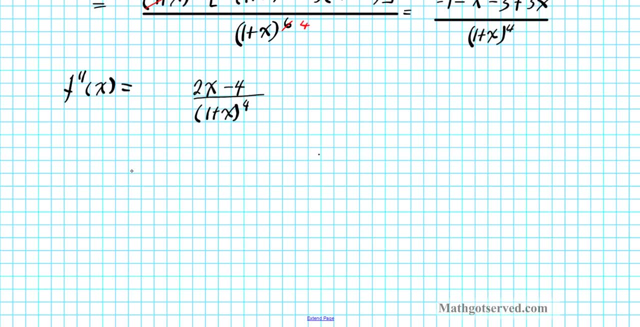 to use that to set up. to use that to set up our um boundary points: okay, our boundary, our um boundary points. okay, our boundary, our um boundary points. okay, our boundary values. so we have values, so we have values. so we have. we're going to look for where f double. 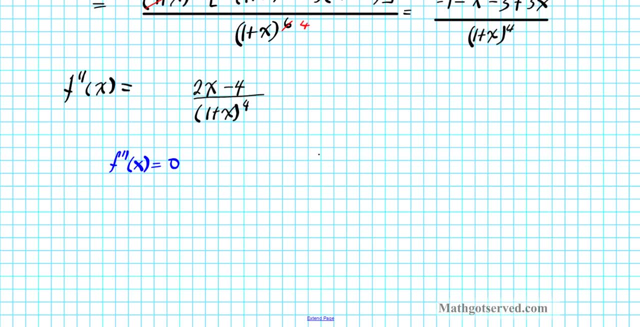 we're going to look for where f double. we're going to look for where f double prime of x, prime of x, prime of x is equal to zero, or where f double prime is equal to zero, or where f double prime is equal to zero, or where f double prime of x does not exist, because this 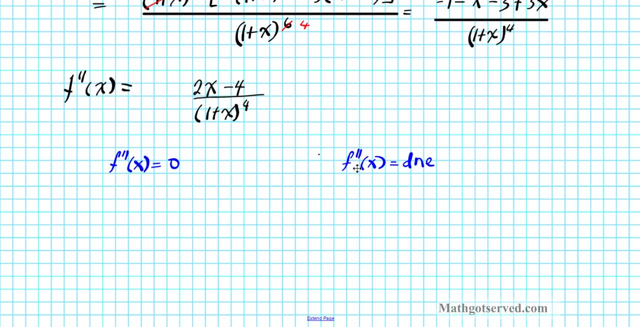 of x does not exist because this of x does not exist, because this are possible, a boundary or values where are possible a boundary or values where are possible a boundary or values where the sign could change. the sign could change, the sign could change. okay, all right, so where is it the second? 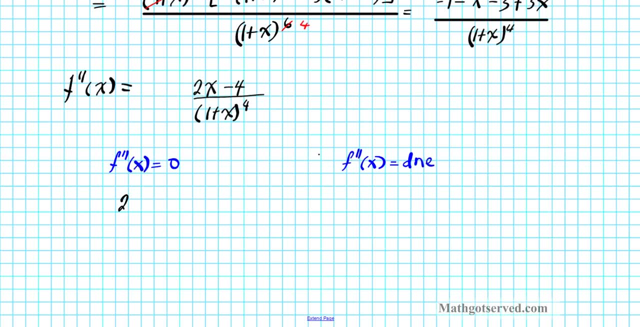 okay, all right. so where is it the second? okay, all right. so where is it the second derivative derivative derivative equal to zero? you said the entire equal to zero. you said the entire equal to zero. you said the entire expression. second derivative expression. second derivative expression, second derivative. set it equal to zero and you solve. 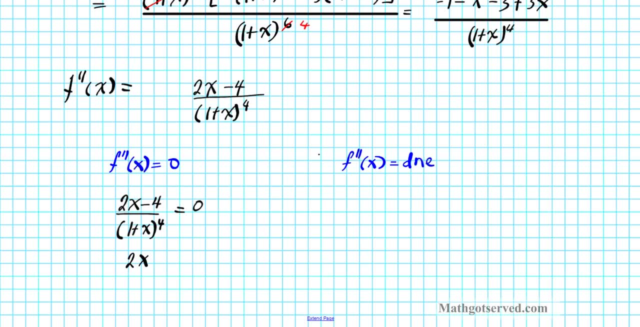 set it equal to zero and you solve. set it equal to zero and you solve: all right. so to solve this, you cross all right. so to solve this, you cross all right. so to solve this, you cross multiply: you have 2x minus 4. multiply, you have 2x minus 4. 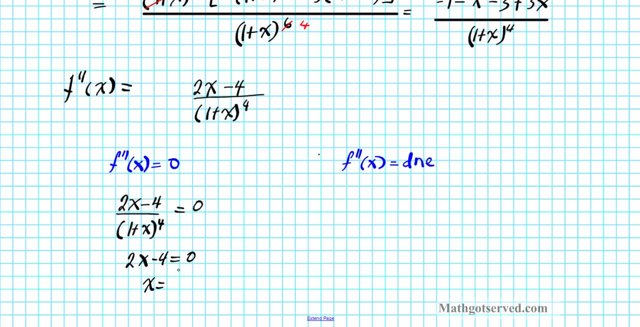 multiply, you have 2x minus 4 equals zero. when you solve for x, you end equals zero. when you solve for x, you end equals zero. when you solve for x, you end up with x up with x. up with x equals four over two. two equals four over two: two. 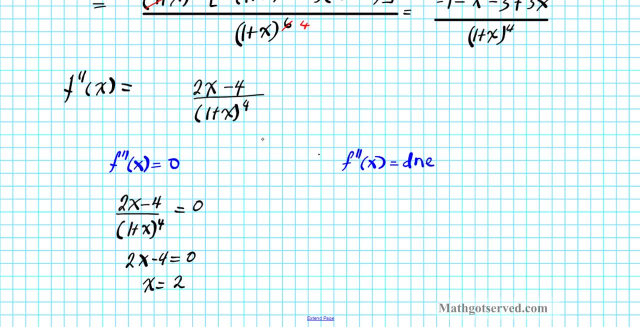 equals four over two. two. when is it undefined or non-existent? when is it undefined or non-existent? when is it undefined or non-existent? um you set the denominator to zero. um, you set the denominator to zero. um you set the denominator to zero. all right, all right. 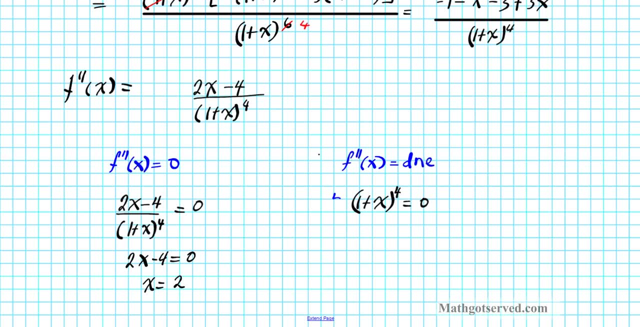 all right, uh, raise both sides to the fourth root. uh, raise both sides to the fourth root. uh raise both sides to the fourth root of both sides, and then we're going to of both sides, and then we're going to of both sides, and then we're going to have um. 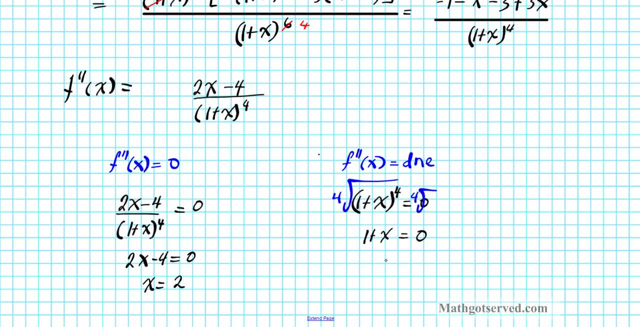 have um. have um: one plus x equals zero, one plus x equals zero. one plus x equals zero, and x equals negative one and x equals negative one and x equals negative one. all right, okay, so what are we going to? all right, okay, so what are we going to? 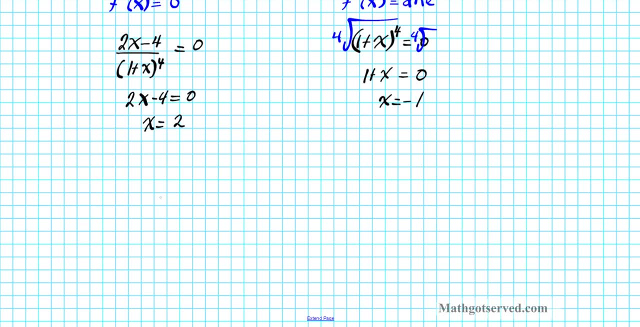 all right, okay. so what are we going to do now? do now, do now. we're going to draw a number line and we're going to draw a number line, and we're going to draw a number line and use the sine of f double prime. use the sine of f double prime. 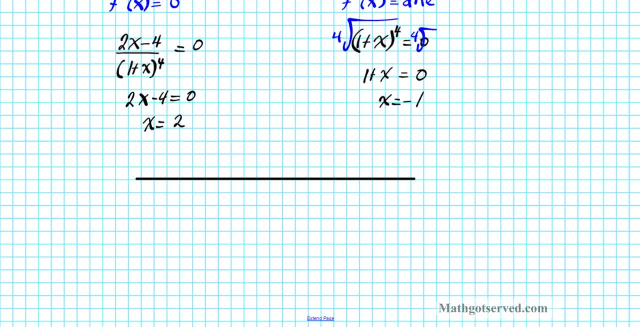 use the sine of f double prime to determine the behavior of f, to determine the behavior of f, to determine the behavior of f. okay, so, okay, so, okay. so we have negative one, we have negative one, we have negative one points, and then we have three intervals points, and then we have three intervals. 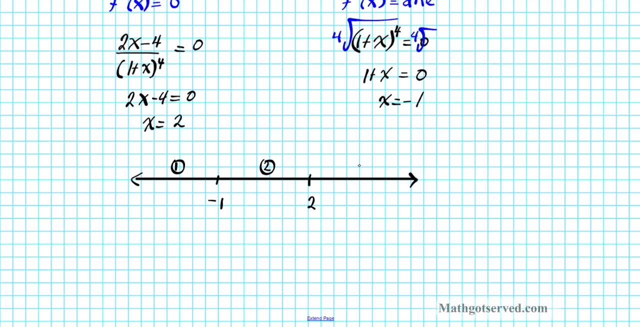 points. and then we have three intervals: interval one interval one interval one interval two. interval three. interval two. interval three. interval two. interval three: now um we want to look for, now um. we want to look for now um, we want to look for the sign, sign of f, double prime on these three. 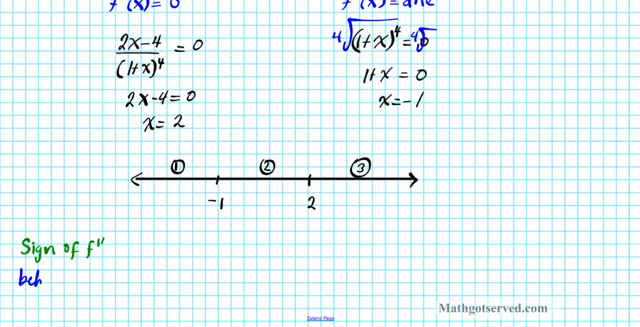 sign of f double prime on these three, sign of f double prime on these three intervals, intervals, intervals, and that will tell us the behavior of f on those intervals of f, on those intervals of f, on those intervals. all right, so let's go ahead. and all right, so let's go ahead, and 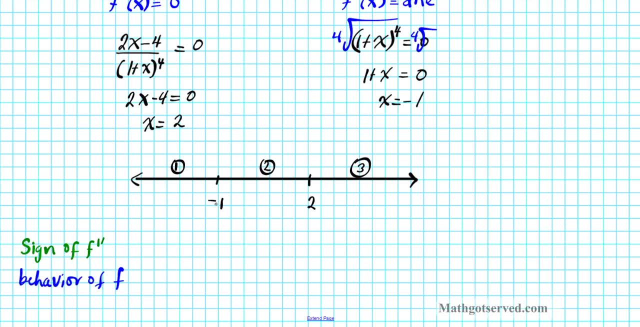 all right. so let's go ahead and partition the interval. so we can partition the interval, so we can partition the interval, so we can clearly see what's going on, clearly see what's going on, clearly see what's going on. so this is the first boundary point. 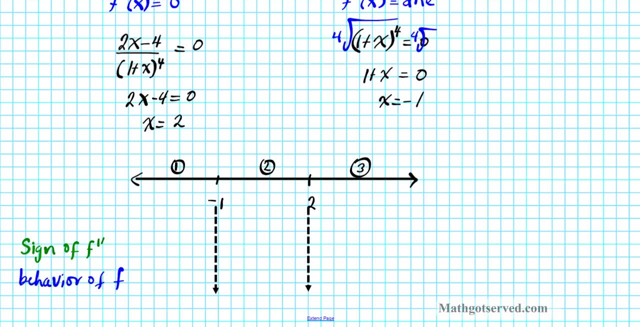 so this is the first boundary point. so this is the first boundary point. where there might be a sign change, it's where there might be a sign change. it's where there might be a sign change, it's not guaranteed, not guaranteed, not guaranteed, and this is another boundary point. if 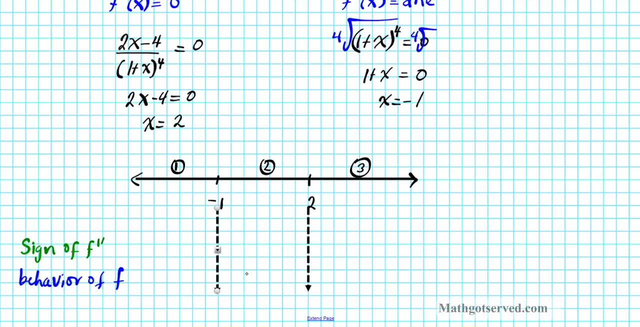 and this is another boundary point- if- and this is another boundary point- if there is a sign change, this is just there is a sign change. this is just there is a sign change. this is just by the way, and the point is by the way, and the point is: 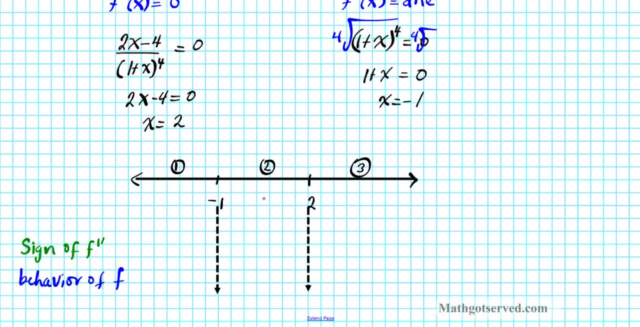 by the way, and the point is: and the function is differentiable at, and the function is differentiable at, and the function is differentiable at that point, that point, that point. the second derivative is defined, then the second derivative is defined, then the second derivative is defined, then you have a the point of inflection there. 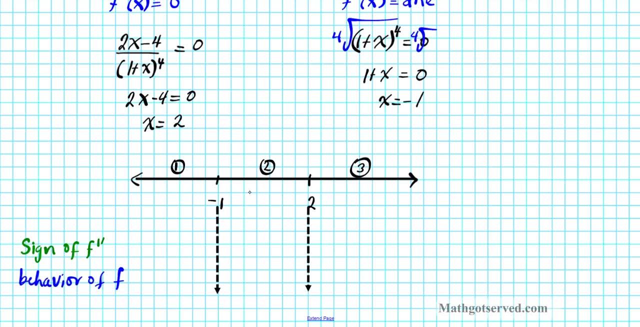 you have a the point of inflection there. you have a the point of inflection there, okay, okay. okay, all right, um, so let's go ahead. all right, um, so let's go ahead. all right, um, so let's go ahead and see what happens. um, for the first interval, we can pick a. 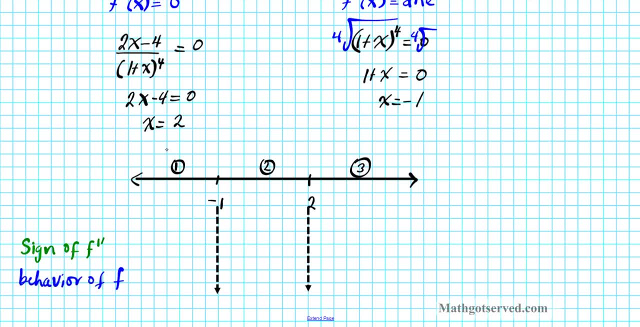 for the first interval, we can pick a. for the first interval, we can pick a value: x equals negative one, and then second x equals negative one and then second x equals negative one and then second interval: we can use zero interval. we can use zero interval, we can use zero. third interval we can use: 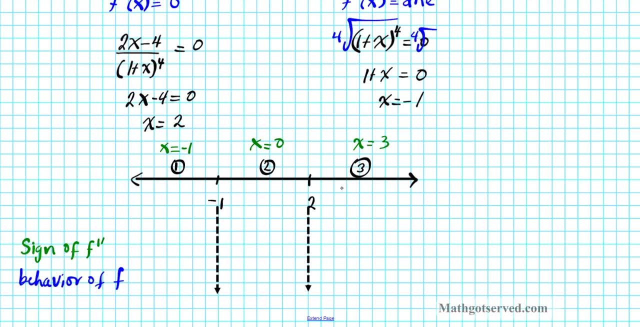 third interval: we can use. third interval: we can use. how about we just use three, all right. how about we just use three, all right. how about we just use three, all right, okay. so let's see what the sign of f. okay, so let's see what the sign of f. 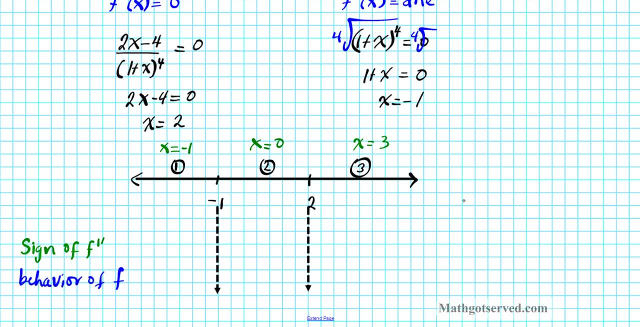 okay, so let's see what the sign of f double prime, double prime, double prime is so for interval one is so for interval one is so for interval one. we're we are testing: x equals negative. we're we are testing x equals negative. we're we are testing x equals negative one. 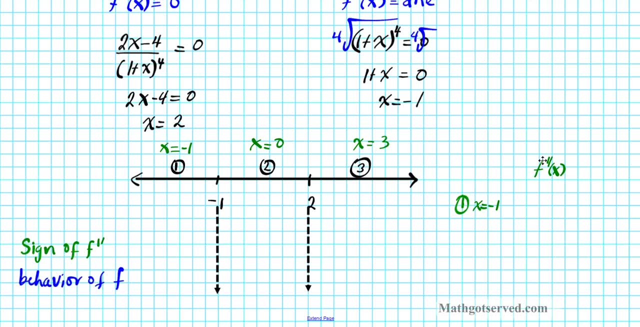 one one. the second derivative f- double prime. the second derivative f- double prime. the second derivative f double prime is is: is is 2x minus 4 over 1 plus x to the fourth. is 2x minus 4 over 1 plus x to the fourth. 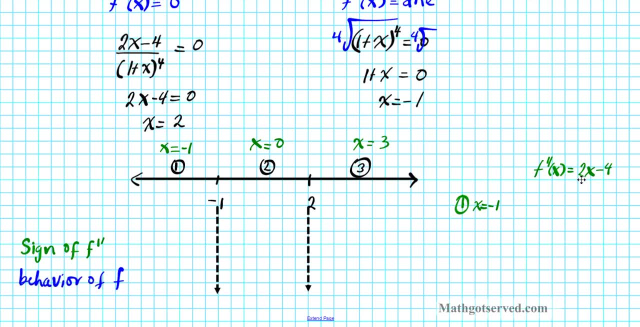 is 2x minus 4 over 1 plus x to the fourth. all i care about is the sign. all i care about is the sign. all i care about is the sign, okay. so i know that if i raise any, okay, so i know that if i raise any, 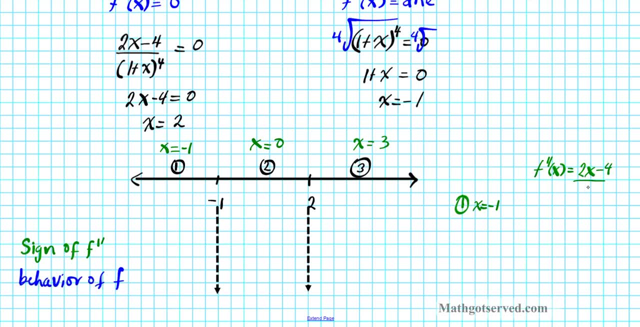 okay. so i know that if i raise any quantity to an even quantity to an even quantity to an even, power is going to be positive. so i don't power is going to be positive. so i don't power is going to be positive, so i don't even need to bother about. 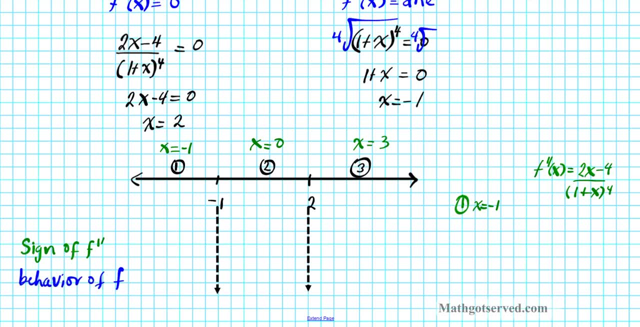 even need to bother about, even need to bother about the denominator, because i know that the the denominator, because i know that the the denominator, because i know that the denominator will always be denominator, will always be, denominator, will always be positive, regardless of what i choose, positive regardless of what i choose. 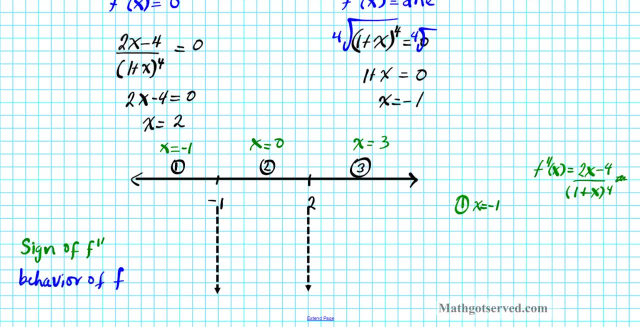 positive, regardless of what i choose. okay, so um on the first interval. okay, so um on the first interval. okay, so um on the first interval. what are we going to have? what are we going to have? what are we going to have? we're gonna um, we're gonna um. 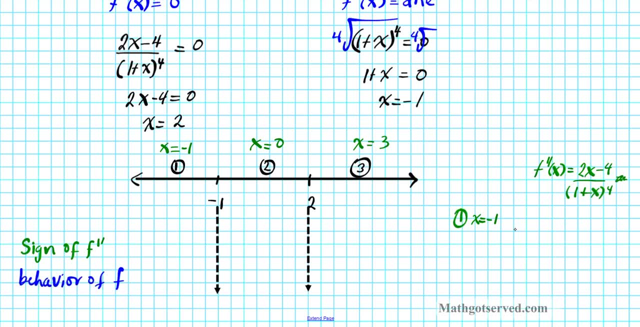 we're gonna um focus our attention on the numerator. if i focus our attention on the numerator, if i focus our attention on the numerator, if i plug in negative one in the numerator, plug in negative one in the numerator, plug in negative one in the numerator. so i'm going to have 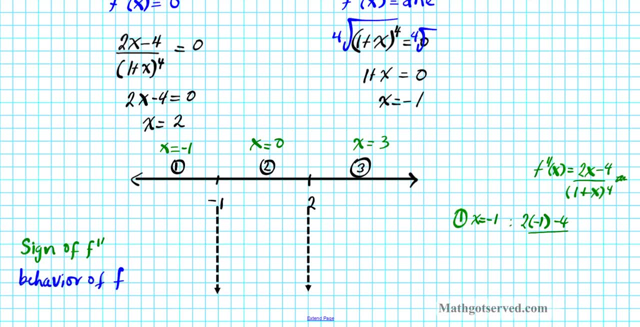 so i'm going to have. so i'm going to have 2 times negative: 1 minus 4, 2 times negative: 1 minus 4. 2 times negative: 1 minus 4, over the denominator which is already, over the denominator which is already. 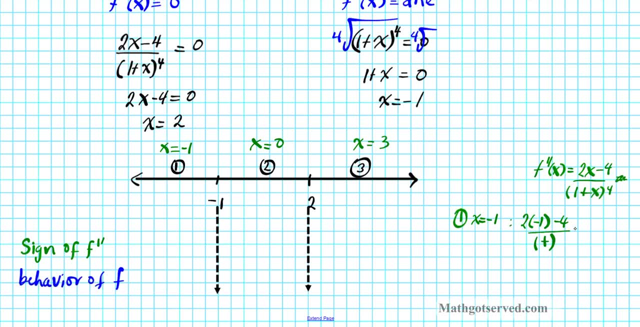 over the denominator, which is already positive, positive, positive. so what is this going to be? it's going to. so what is this going to be? it's going to. so what is this going to be? it's going to be be a negative over a positive, which is negative, all right. so it's going to be a negative sign. 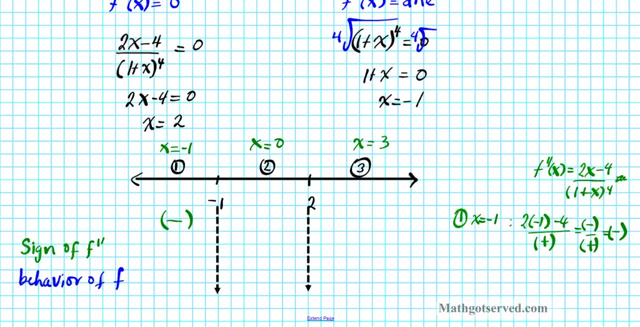 which is all i care about. so it's negative. on this interval: all right, interval two x equals zero. we're gonna have two times zero minus four over a positive number, four. all right, that's going to give us a negative result divided by positive, which is negative. 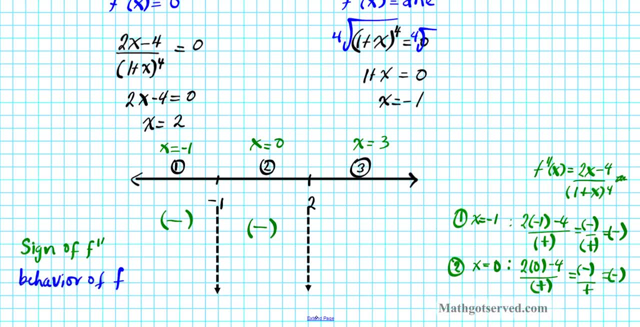 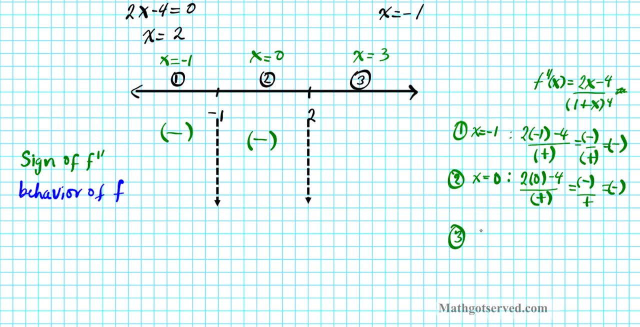 again. so we have a negative sign on interval two. and then, lastly, we have f: 3 x equals three. we're going to have two times three minus four over. a positive number which yields two times three is 6 is bigger than this, so it's going to be positive. divided by positive is positive, so we 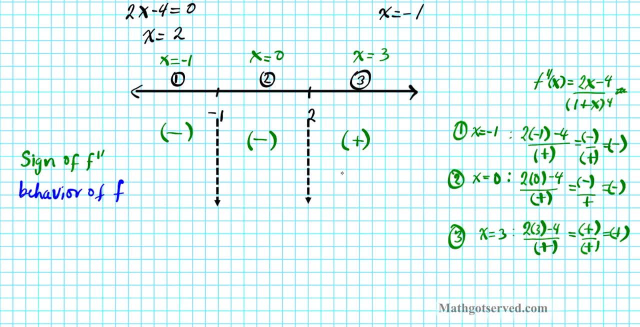 have a positive second derivative sign on interval um number three. okay, let me line my signs up properly. it's all over the place. so we have sign of the f double prime is negative, negative, positive. so what does that tell us about the behavior of f, if it remember the rule, if um. 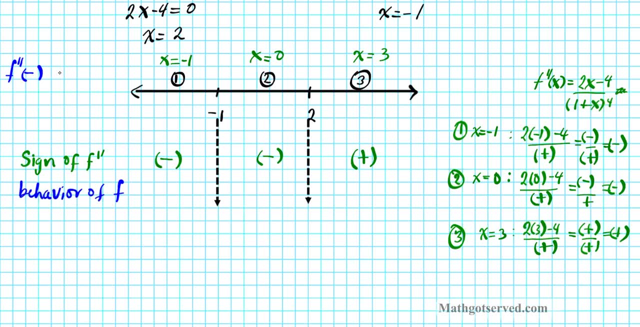 f double prime is negative, f is going to be what? concave down? right. and if f double prime is positive, f is concave up. talked about this earlier. so it's concave down, concave down, concave up, all right, so let's go ahead and write down our answers. so f is concave up.